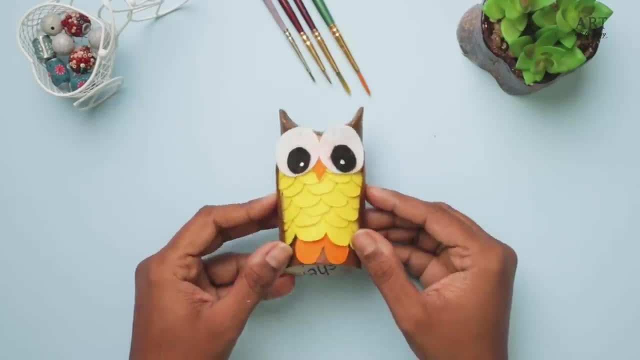 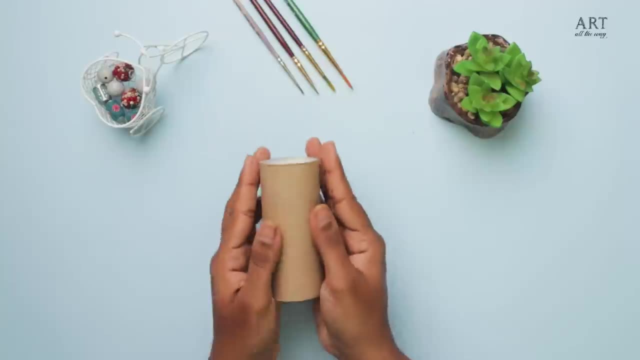 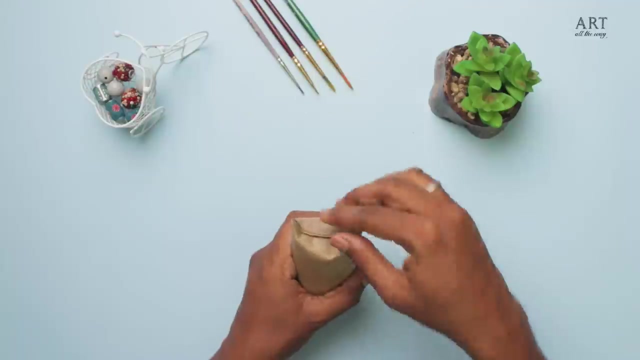 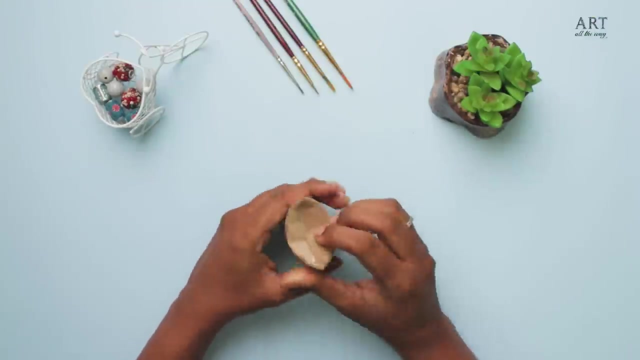 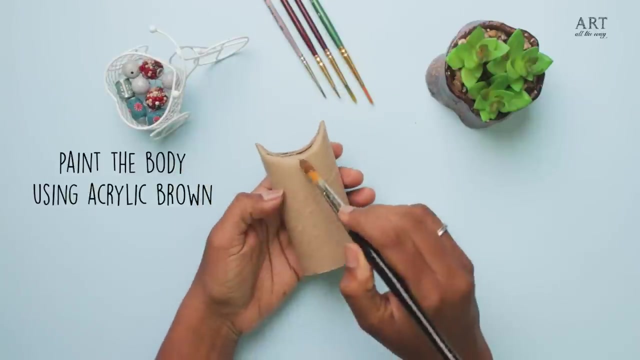 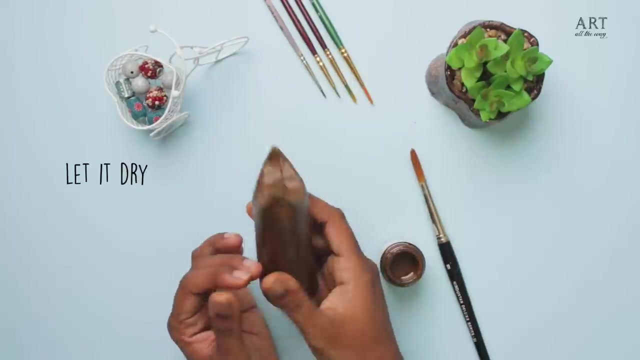 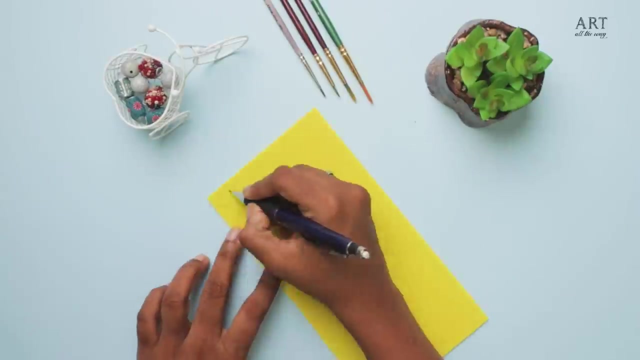 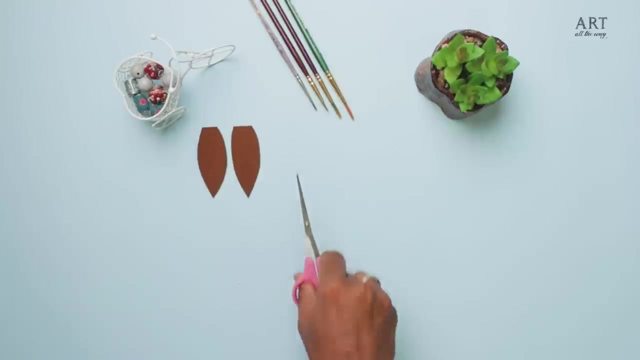 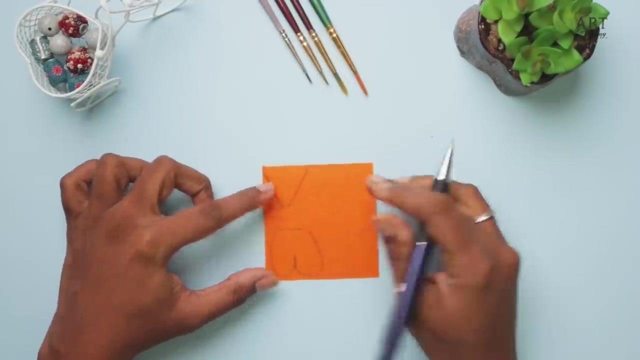 Hello everyone. this is Thomas. I'm a person who likes creating videos for YouTube. I also try to post videos that are easy to follow. I make many things and always want to share them with you. You will always be there, Always alone. You will always be there. 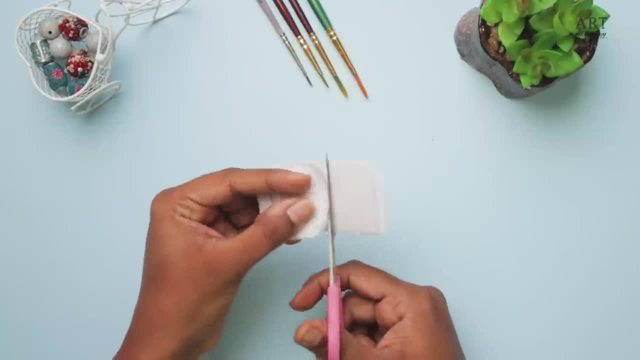 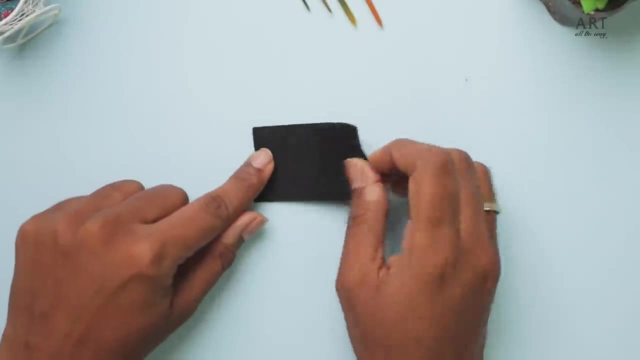 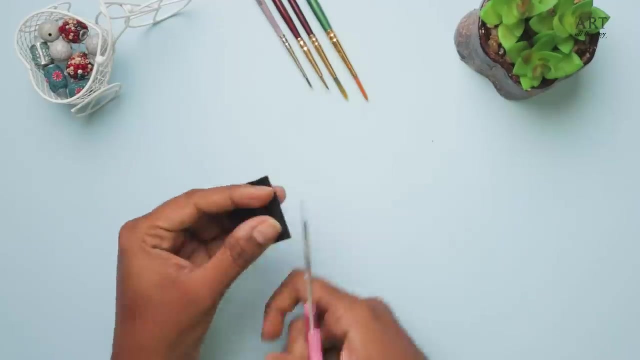 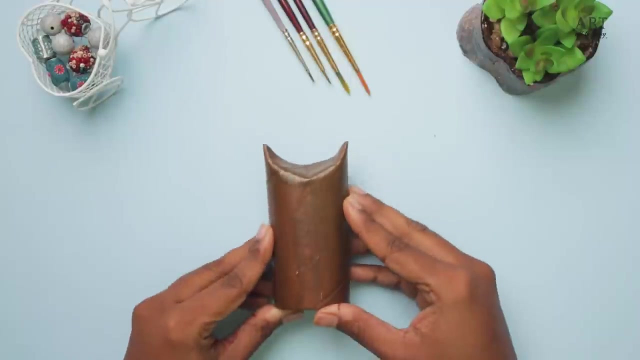 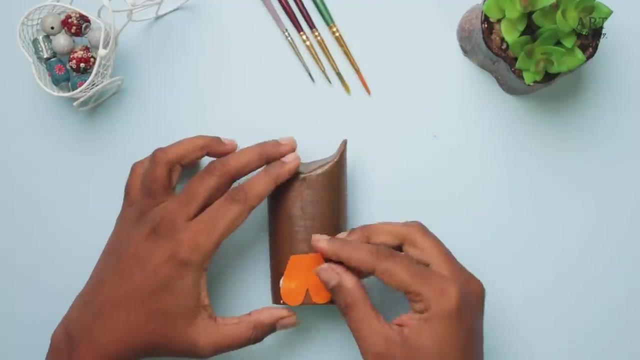 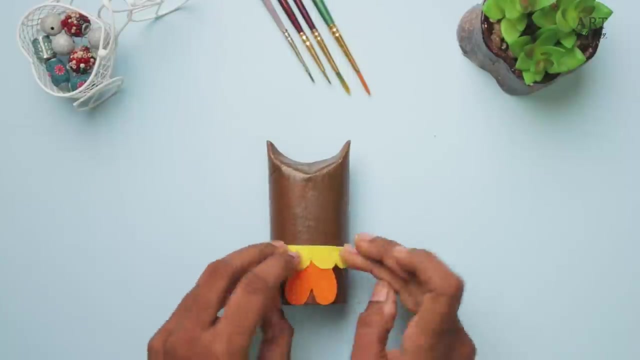 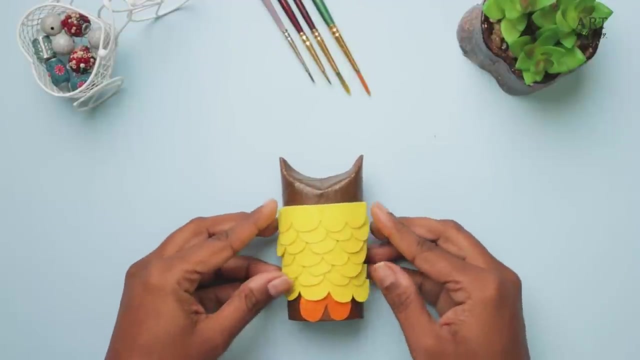 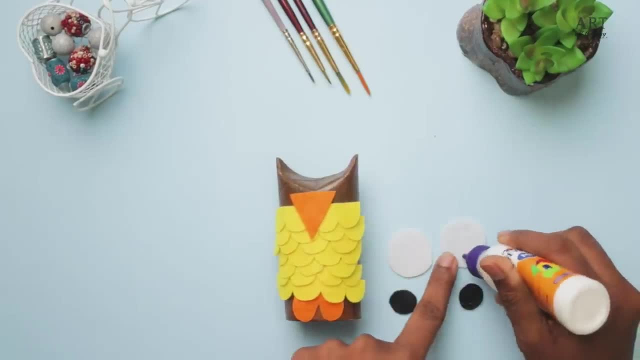 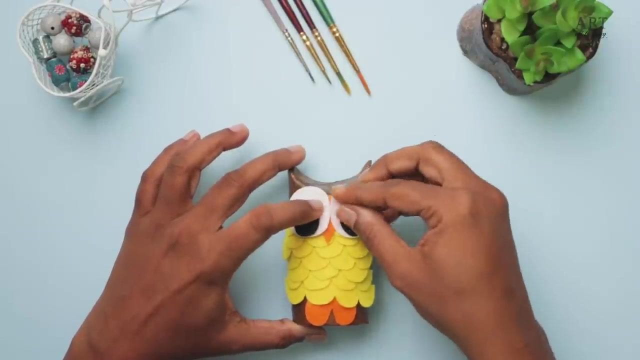 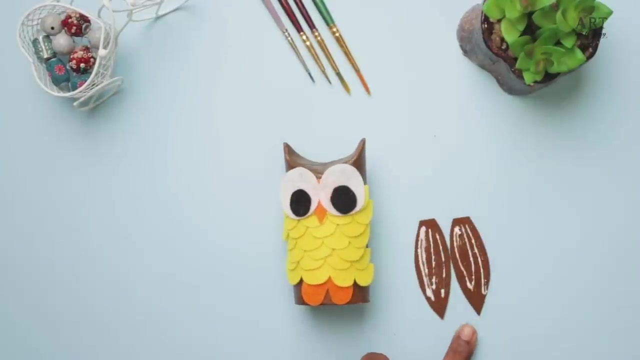 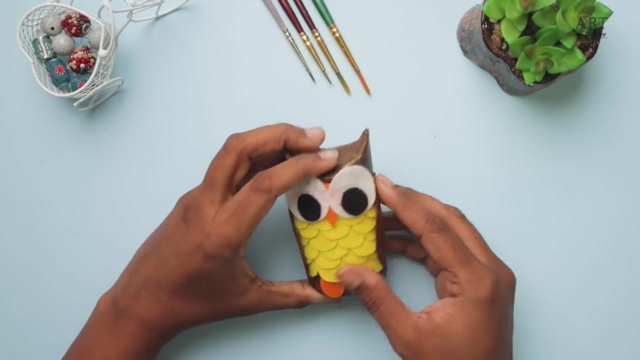 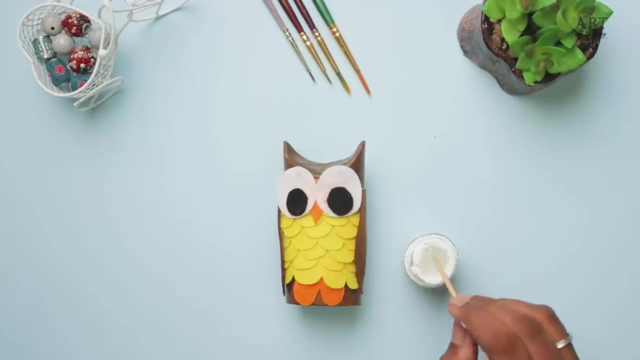 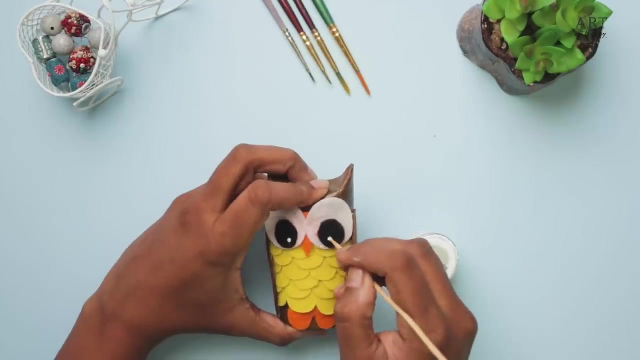 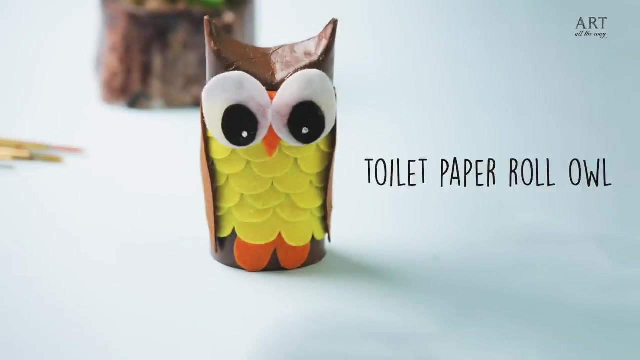